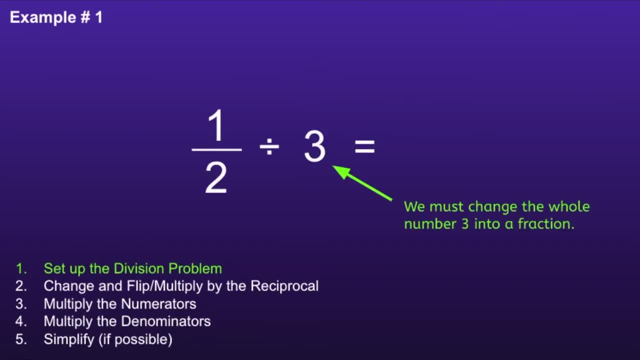 The next step is to change the whole number three into a fraction. We can change any whole number into a fraction by giving it the denominator of one. This moves us on to step number two: Change and flip or multiply by the reciprocal, And these are the steps to divide fractions. 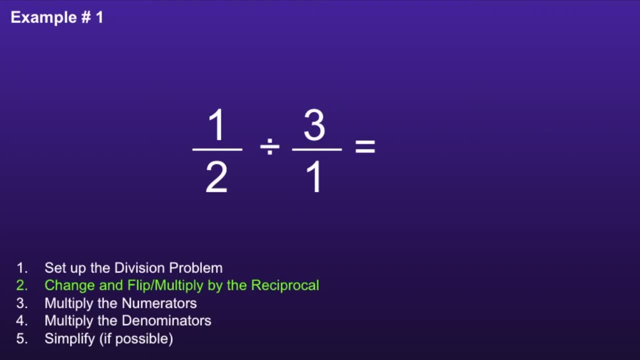 And what it means is we want to change the division sign to a multiplication sign and take the reciprocal of the second fraction, Which means switching the numerator and denominator, So we can change the numerator and denominator, So three over one will become one over three. 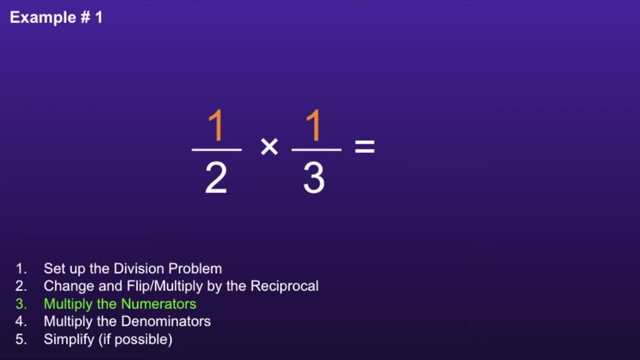 Moving on to step number three, Multiply the numerators. One times one is equal to one. Step four: Multiply the denominators: Two times three is equal to six. And finally, step number five: Simplify if possible. Since we cannot simplify the fraction, we can use a little more detail. 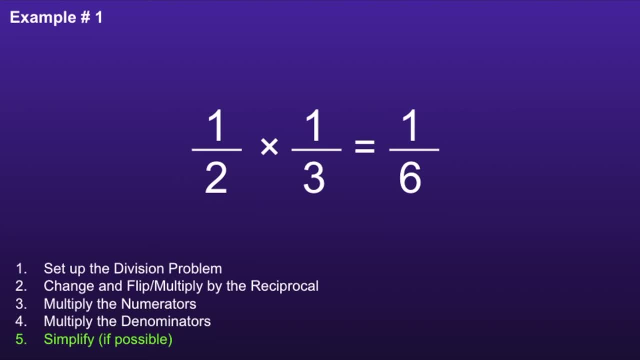 Why 1 over 6, we are done. So 1 half divided by 3 is equal to 1. sixth Example, number 2.. 2 fifths over 3 fourths. Step 1 is to set up the division problem. We know it's going to be a division. 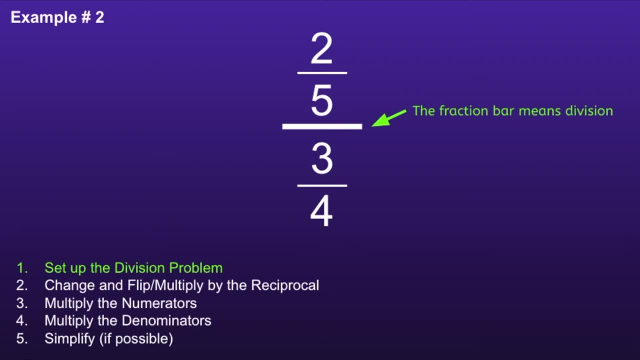 problem, because the fraction bar means division, So we can set this up as 2 fifths divided by 3 fourths. This moves us on to step number 2.. Change and flip or multiply by the reciprocal. In order to do this, we change the division sign to a multiplication sign and take the reciprocal. 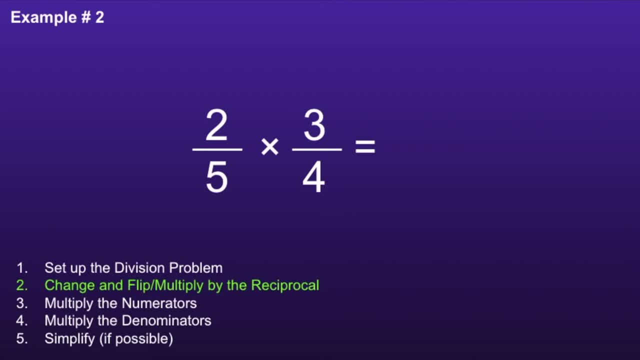 of the second fraction, which means switching the numerator and denominator, So the fraction 3 fourths becomes 4 thirds. Step 3. Multiply the numerators. 2 times 4 is equal to 8.. Step 4. Multiply the denominators. 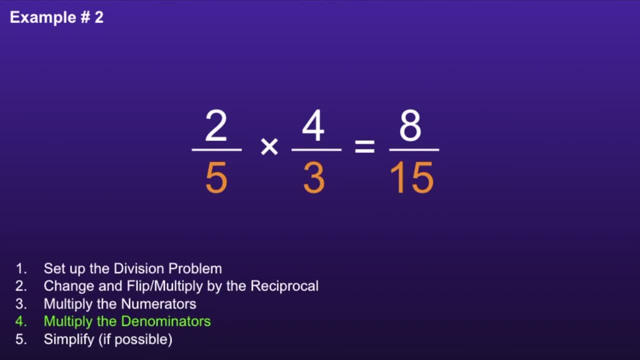 5 times 3 is equal to 15.. And finally, step number 5.. Simplify, if possible. Well, we have to determine if there are any common factors between 8 and 15.. If I think of the factors of 8, it would be 1,, 2,, 4, and 8..